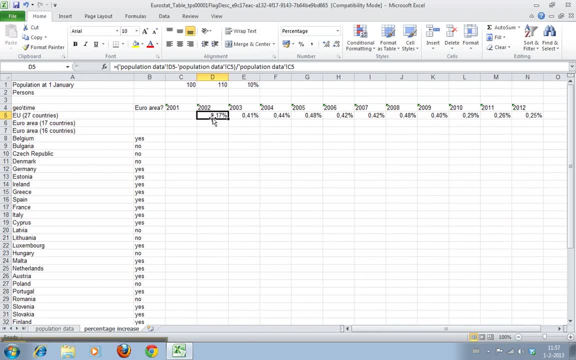 minus d, that one. oh, this is actually proper. this is right away. um, because it always has to take the total population of last year, the difference between this year and last year and divided by last year. so this is actually good. i was still. i had a for a minute. i thought we had to do complicated. 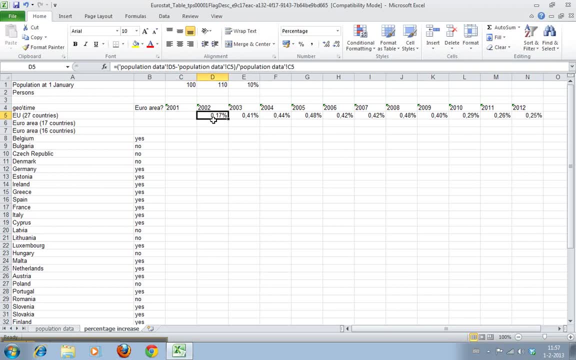 stuff with cell references and fixed and relative cell references, but we don't actually, so we only have to calculate this value. but actually that's a bit um, yeah, because now it tries to calculate stuff with b5 and there's nothing in b5. so this is all c, because this is this. this is the only year that has to compare to itself. 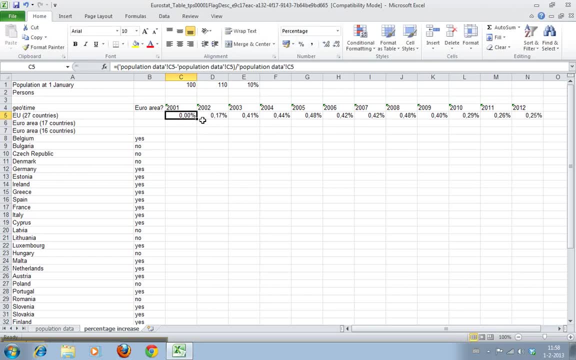 and it should be a hundred percent. oh no, it should be zero. yeah, it's actually because the last need your access to this data and it should be a million on all of the target cells. so this was totally a много. and to take this data simply to and then, in theュ, take it to the 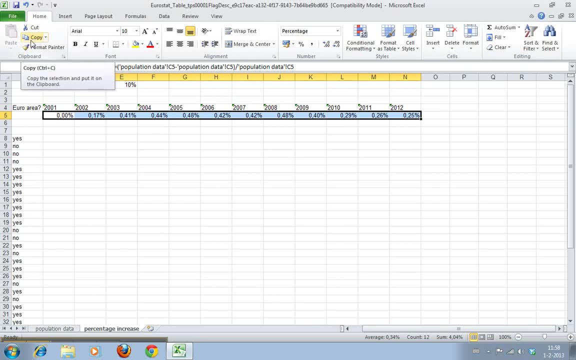 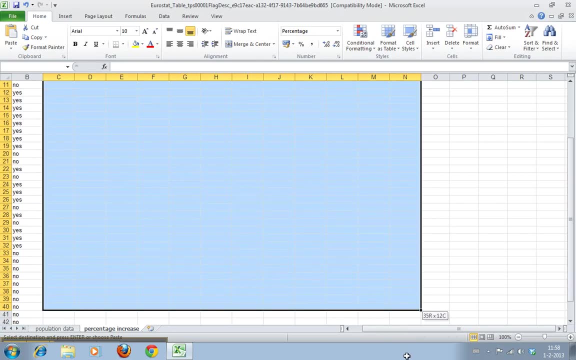 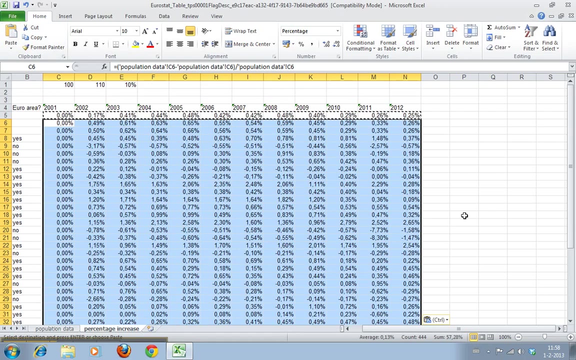 smashing unboxer and so, and it has all that value and you can see that qt tidy data is valid, as you see as well. and so now take in the other hundred percent of the Boston value and put it on the c元 as so pg. 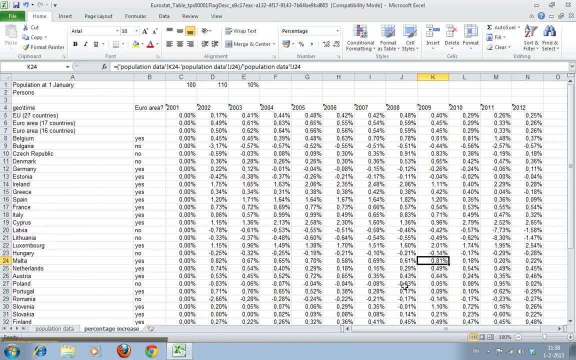 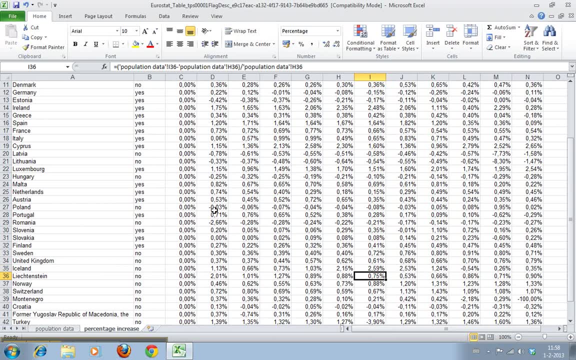 and there we have it and, as you can see, it's still a large data set, but it's a bit more meaningful. you can see, hey, this country is always dropping in. this country- which would country is that? that's Romania and Slovenia- is almost always, except for 2008- it's always increasing. so this is a bit more. 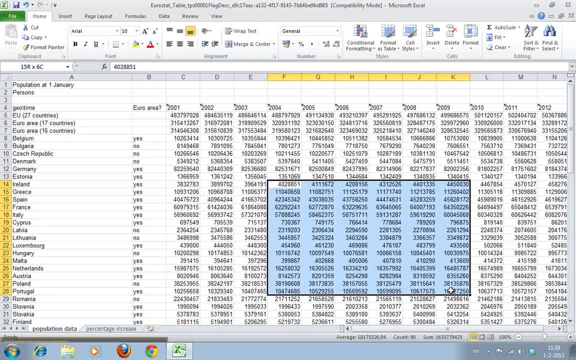 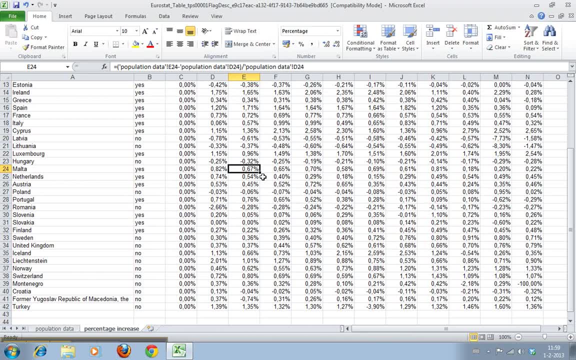 meaningful than this whole big junk of numbers. all right, and of course, we can use this data in graphs, in charts. we can also do some formatting tricks with it, which will be next video. and, yeah, you can. you could even calculate average percentage increases and everything you want with it. and the trick is because